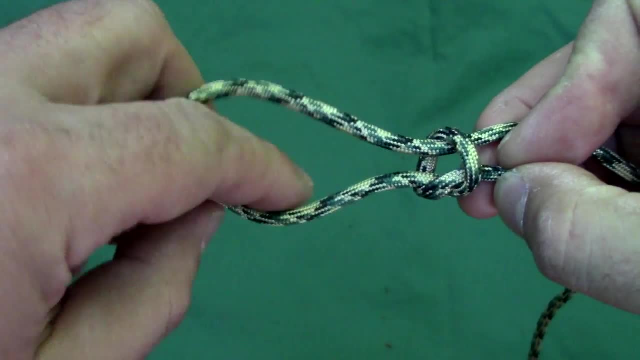 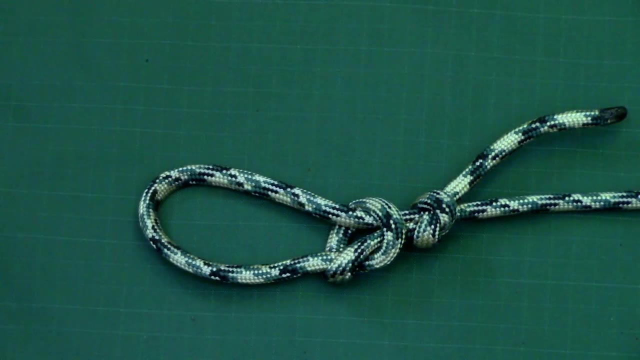 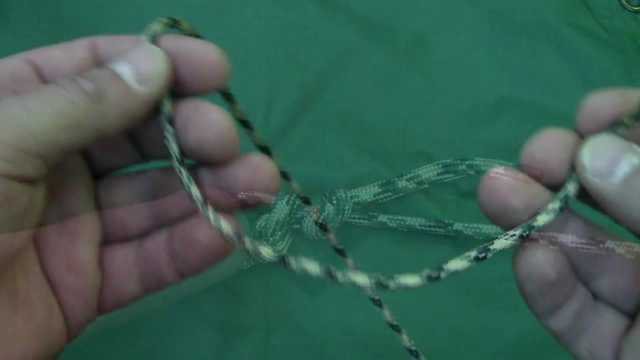 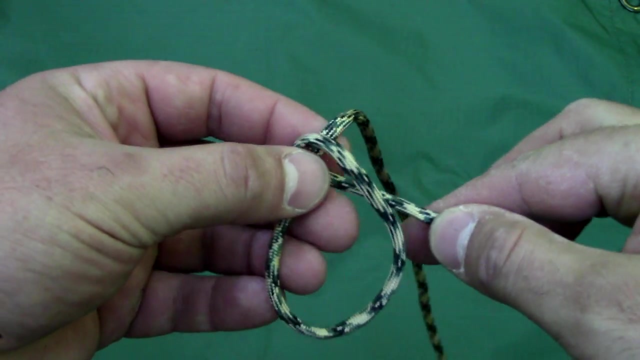 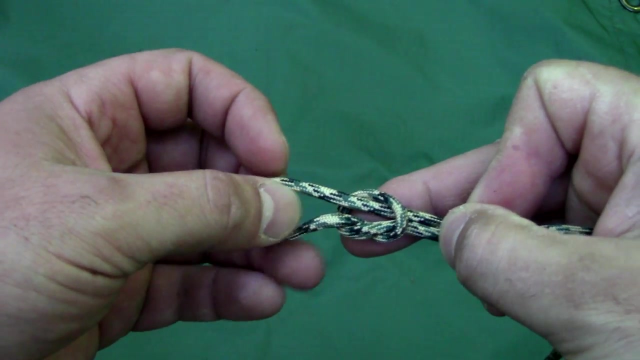 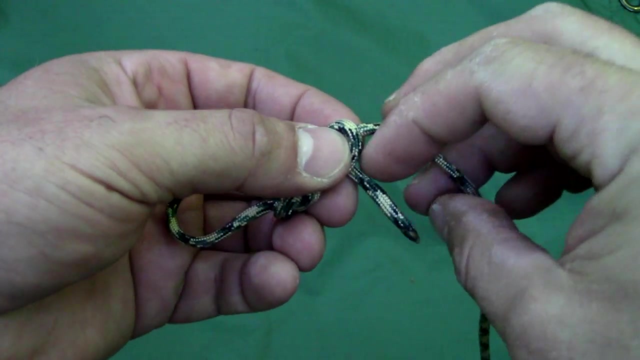 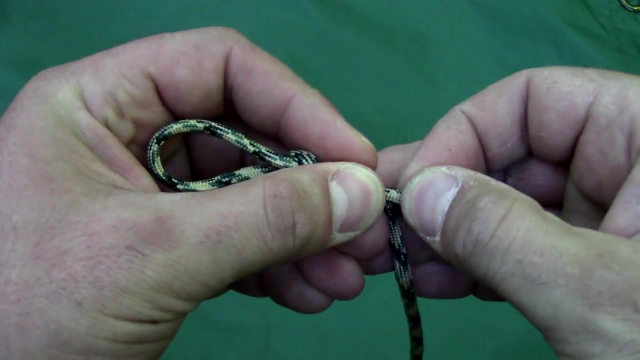 A jam knot is a combination of a slip knot and stop knot. that will also tighten when the line is pulled. A basic bowline creates a perfect non-slip loop. A basic bowline creates a perfect non-slip loop. A basic bowline creates a perfect non-slip loop. 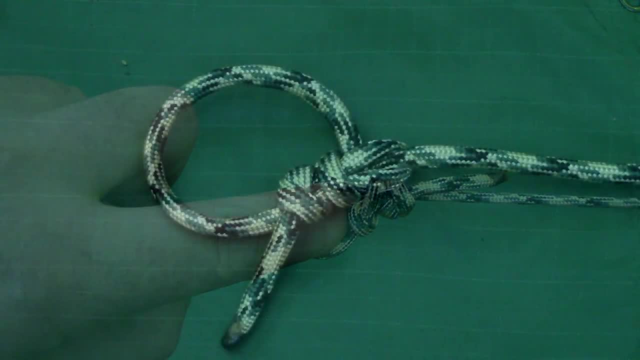 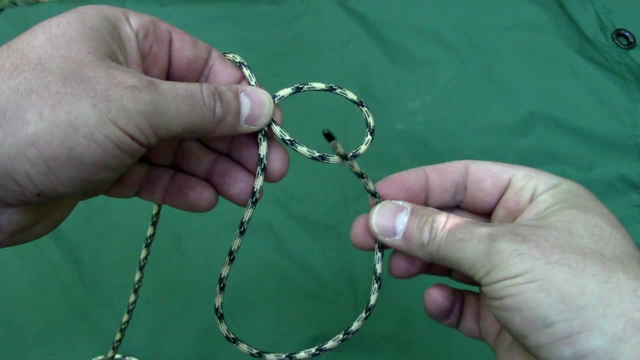 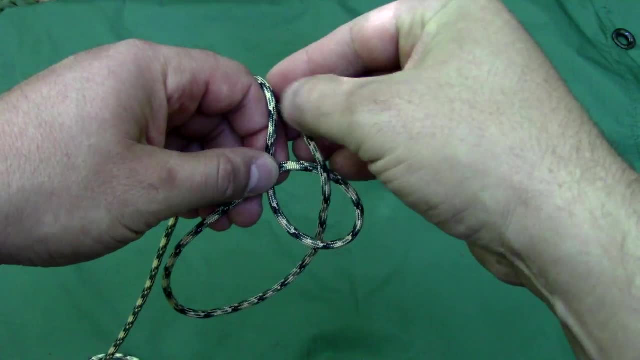 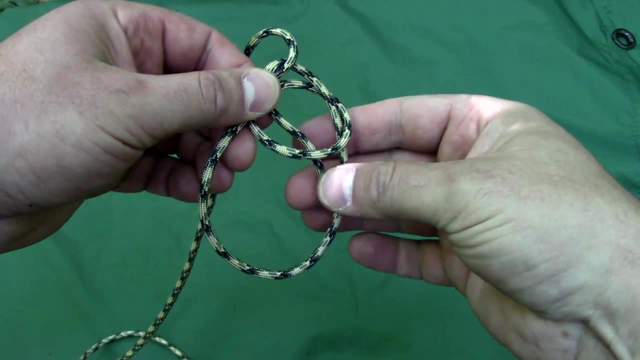 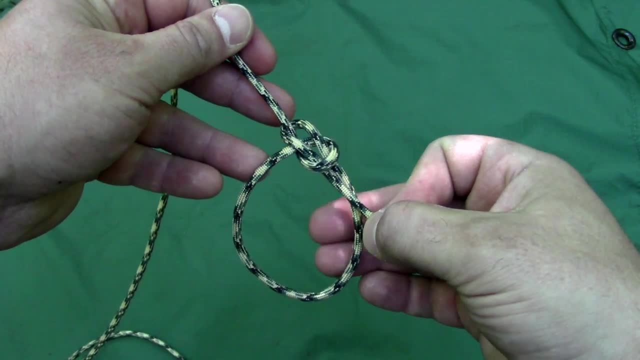 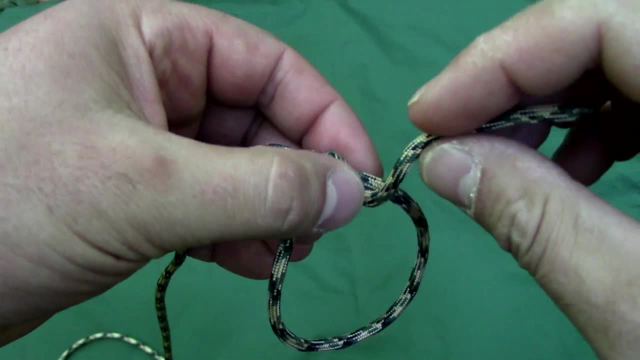 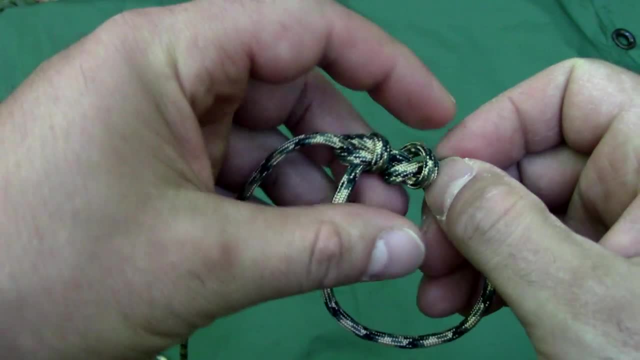 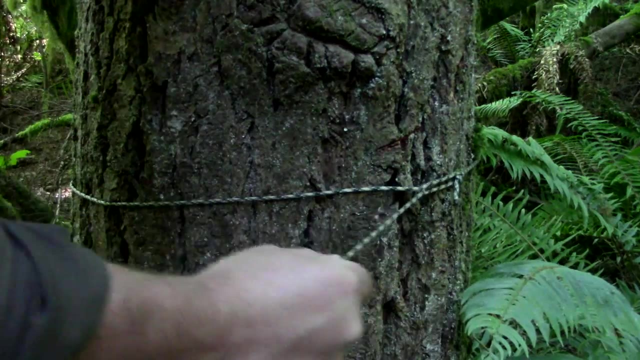 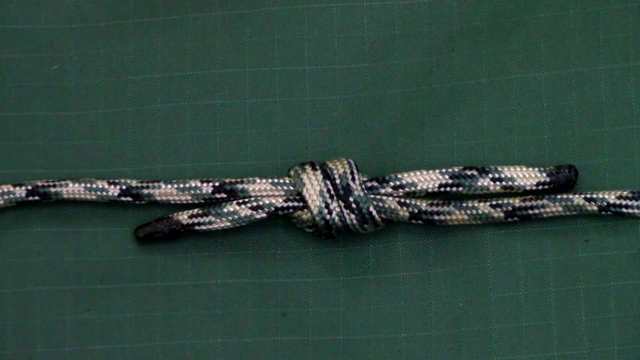